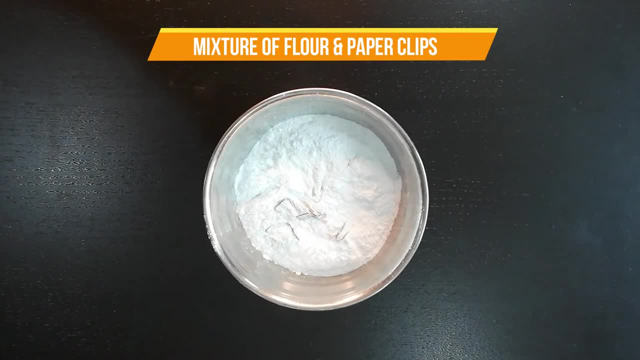 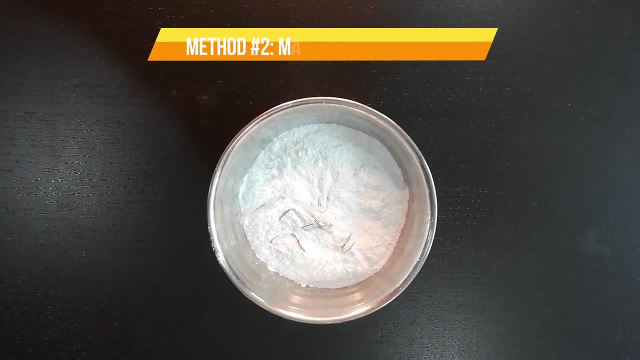 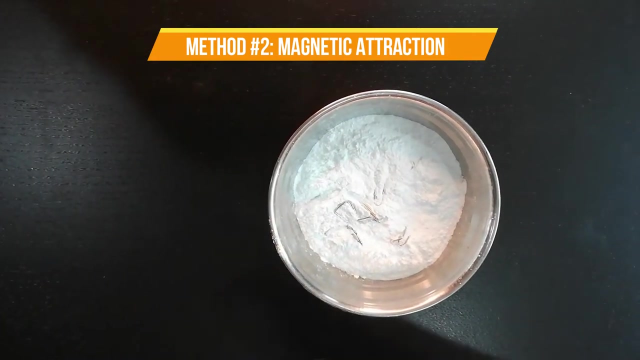 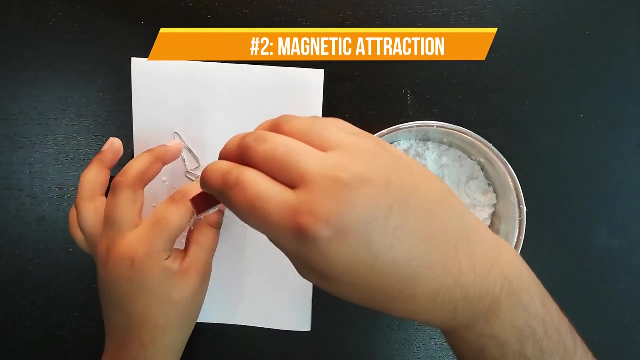 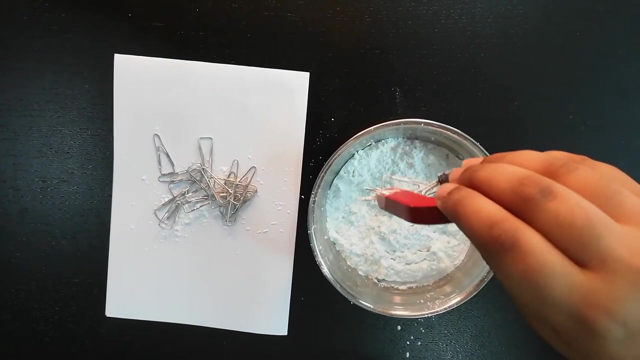 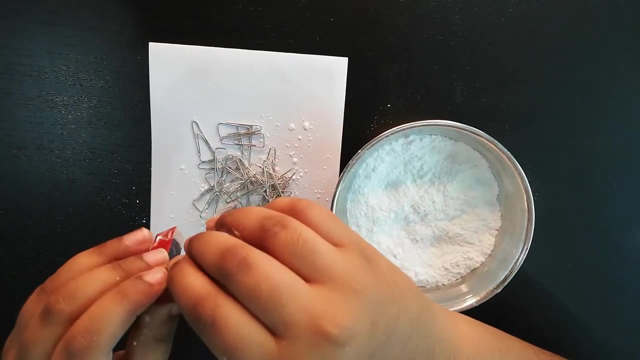 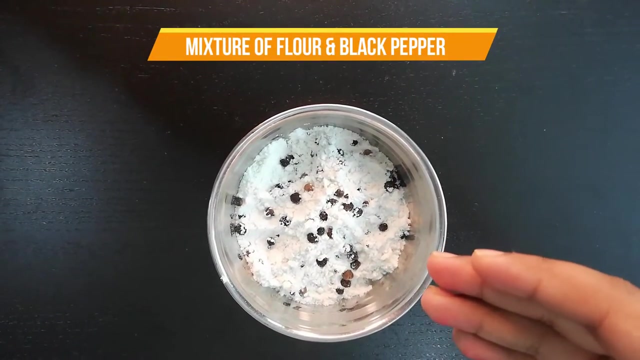 mixture of flour and paper clips. One easy way to separate them is through magnet. Magnetic attraction is used to separate materials that can be attracted by a magnet. The clips are separated from the flour. This is the mixture of black pepper and flour. The best method to separate them is through sieving. It is because you are trying to separate. 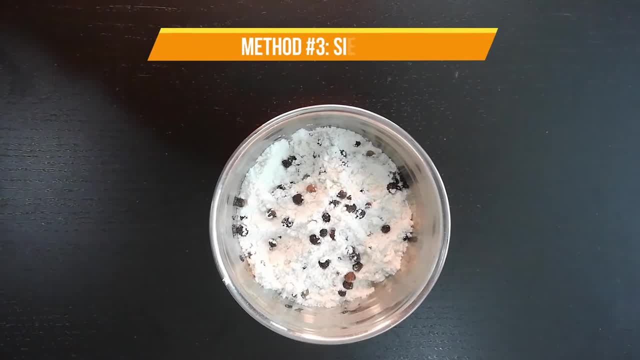 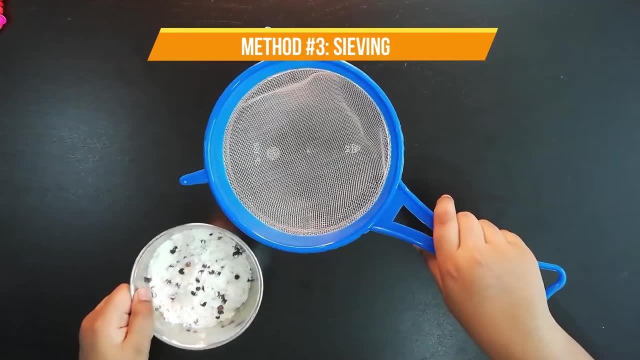 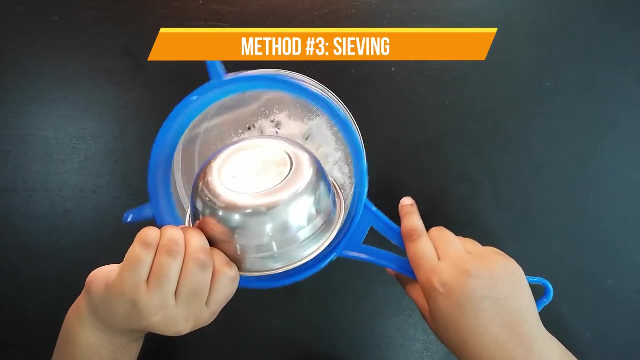 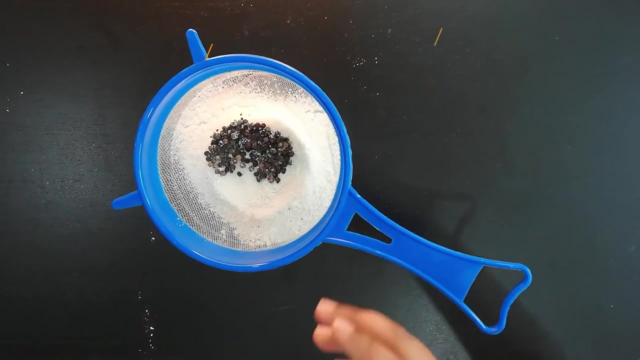 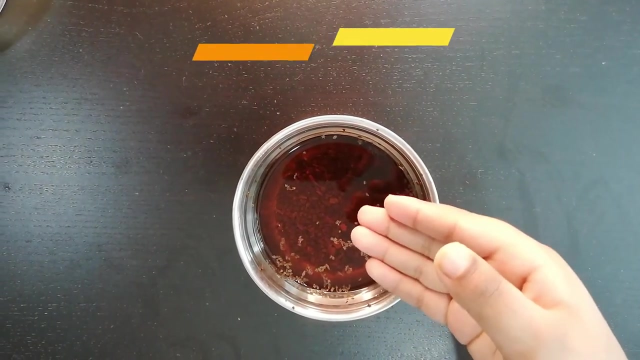 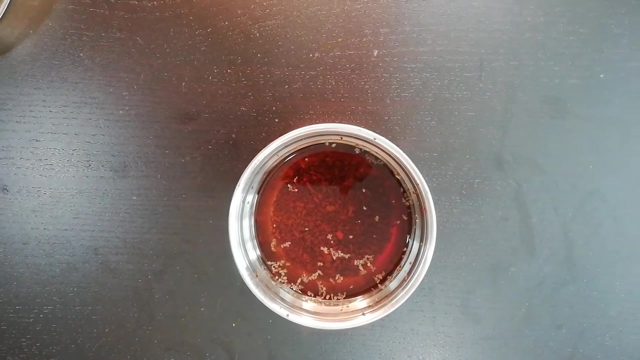 fine sized material and large sized material For sieving. we need to use the sieve. As you can see, the pepper is already separated from the flour. This is the mixture of crushed tea leaves and water. The best way to separate them is through filtration. This is because one of the substance is heavier than the other. 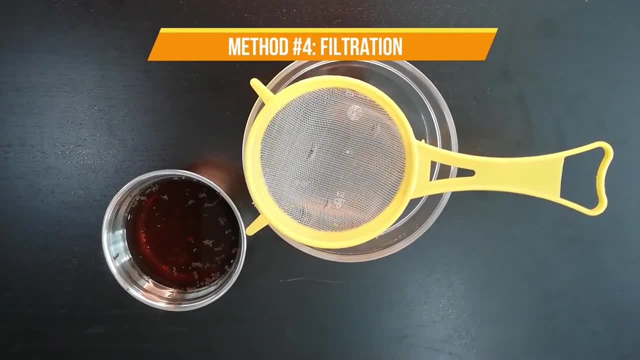 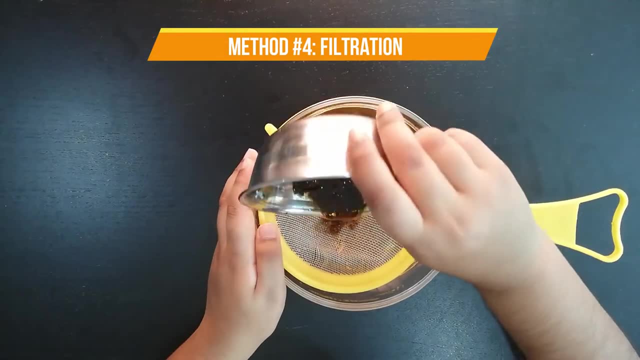 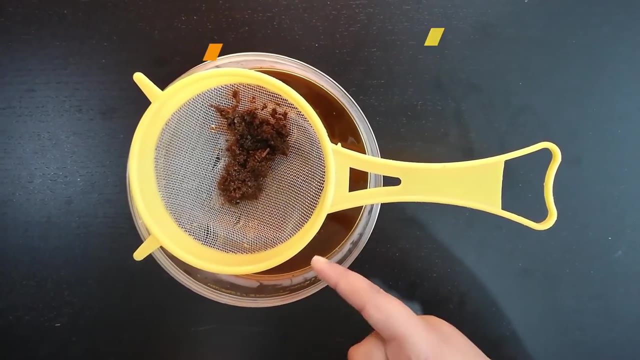 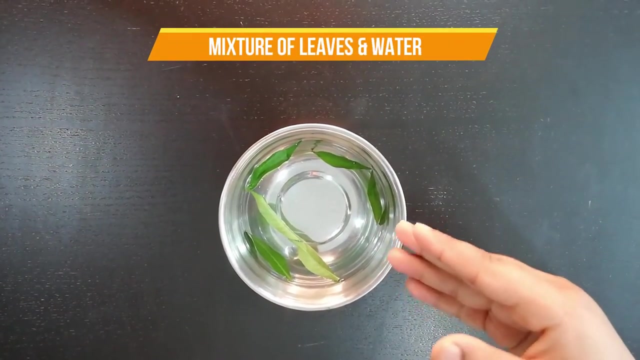